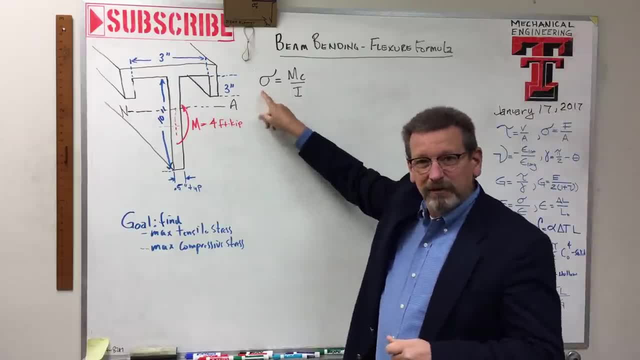 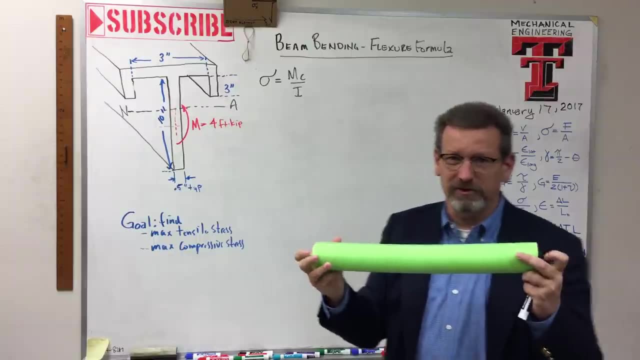 semester. So what does that mean? What kind of stress is sigma? Remember that's normal stress, That's the stress that makes this beam longer or shorter. right, A compressive or a tensile stress? okay, Well, what's happening On the top? what do I have? Compression, right, And I'm 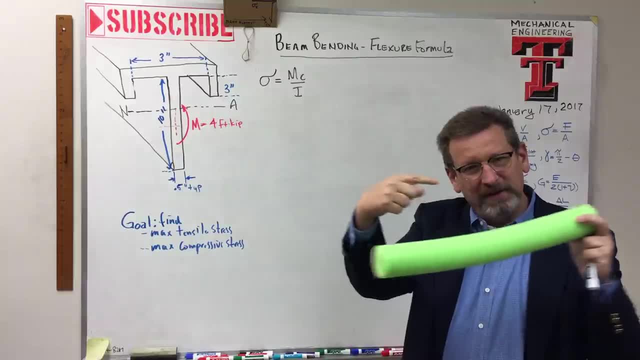 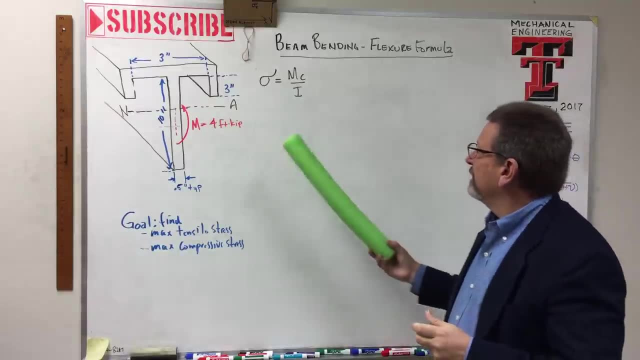 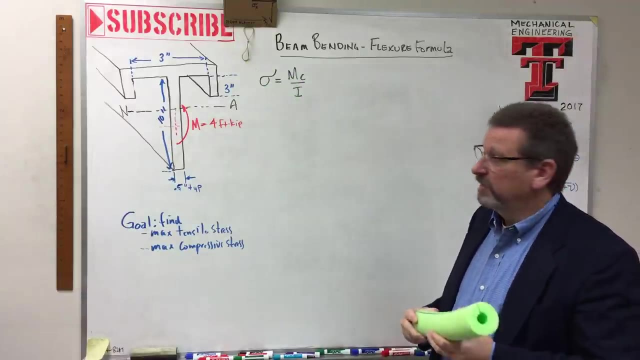 being squeezed together. So the top, there's stress due to those fibers being in compression. On the bottom, there's stress due to those fibers being pulled apart in tension. okay, So that's where this comes in. So, on the top of this beam, I'm going to have compression, I'm going to have 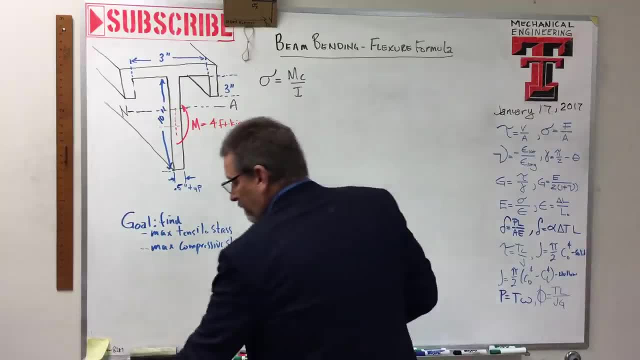 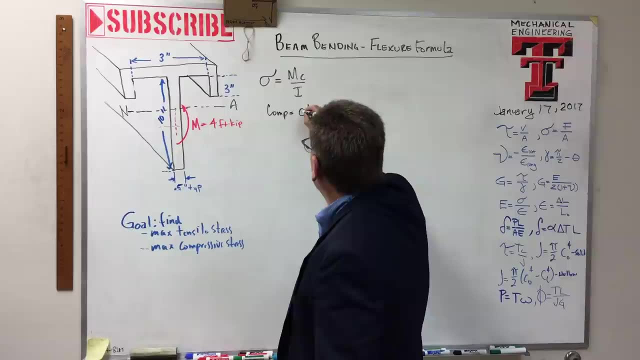 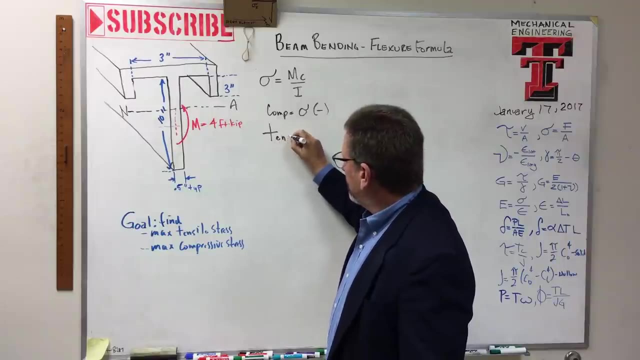 a tension from the compression and, on the bottom, from tension getting longer. And remember this, that compression is going to have sigma is going to have a negative sign. And then tension. what does tension start with? A positive sign, right? Sigma is going to be positive, right? So 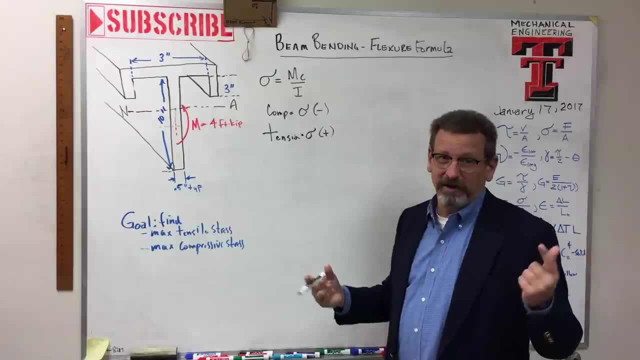 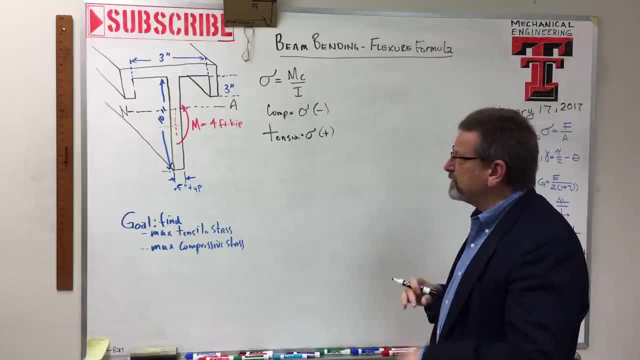 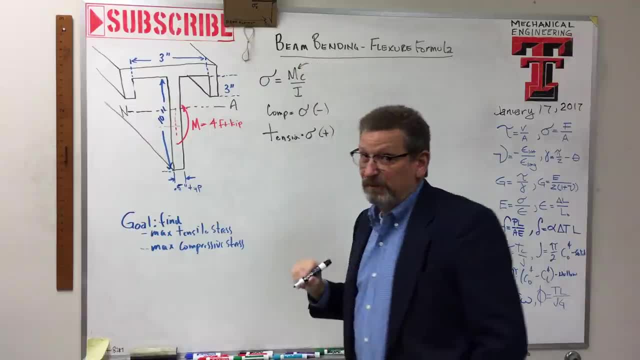 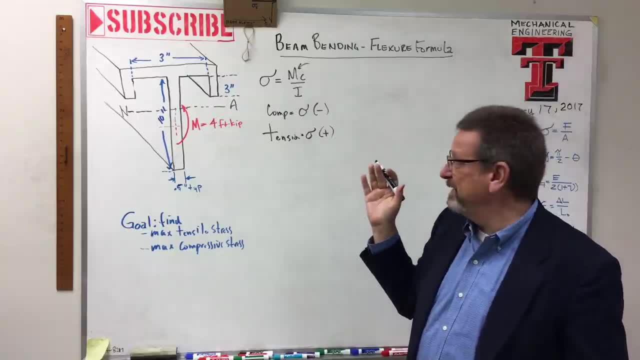 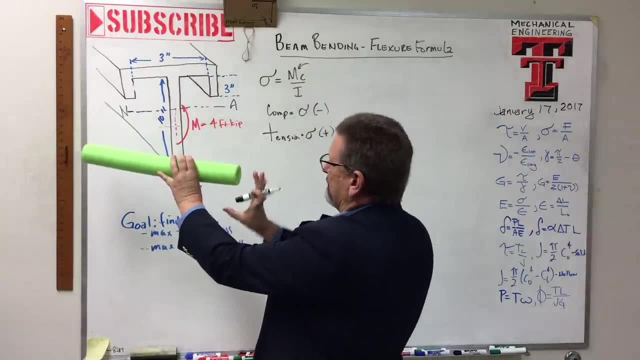 have to. we can draw a shear moment diagram. We can tell you what m is at any point on the beam. On this problem. they say that you know, here's the beam. They have this moment like that, right, Something is twisting its four foot kips, so that that moment is twisting it like so okay, So we 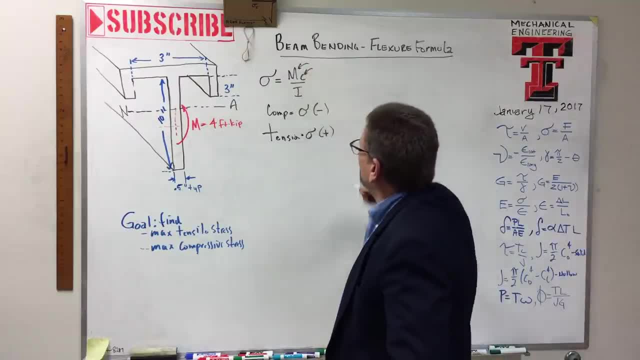 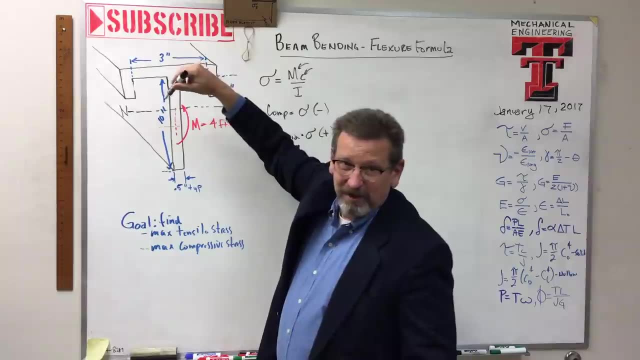 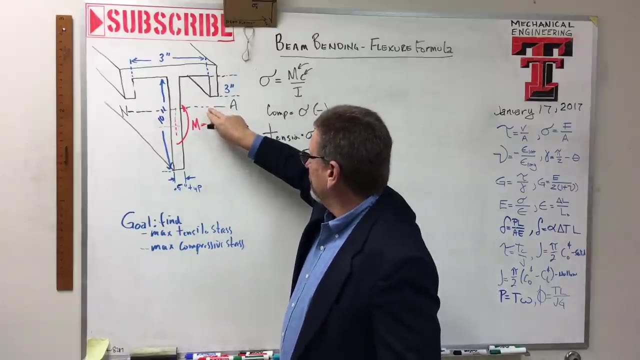 already know the bending moment for this one. What is c? Well, that is the distance from the neutral axis to the point I'm interested in. and in this point they say: find max tension. So where's maximum going to happen? Well, it's zero here and it starts increasing, increasing. 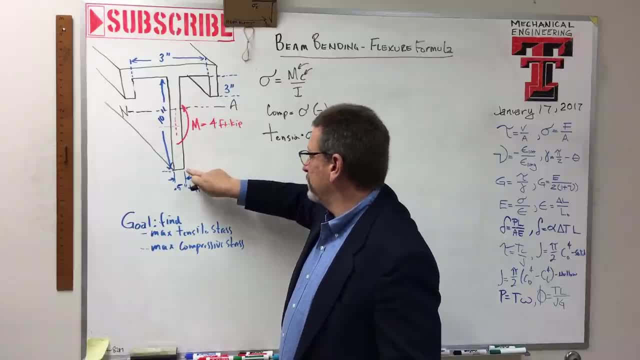 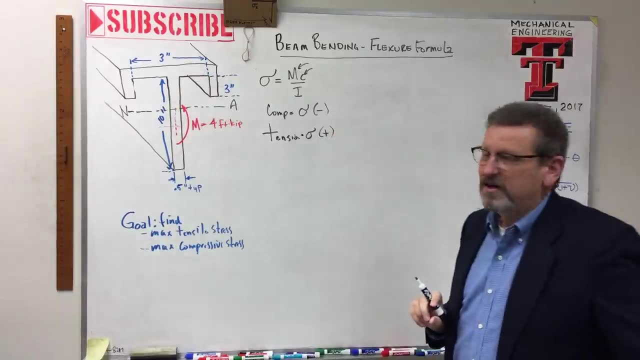 increasing. so the max is going to be on the very outside of the part. So this is max, or that is max, right? This is max for compression, This is max for tension. okay, So c is a distance, okay. 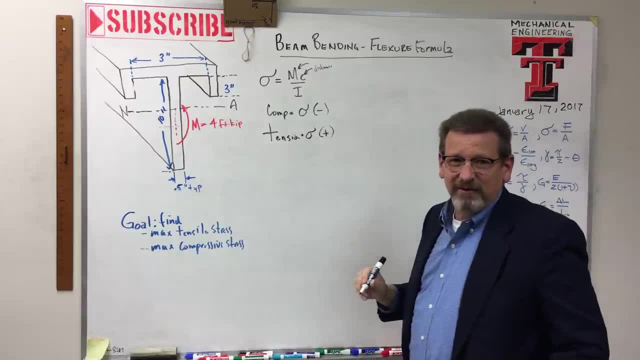 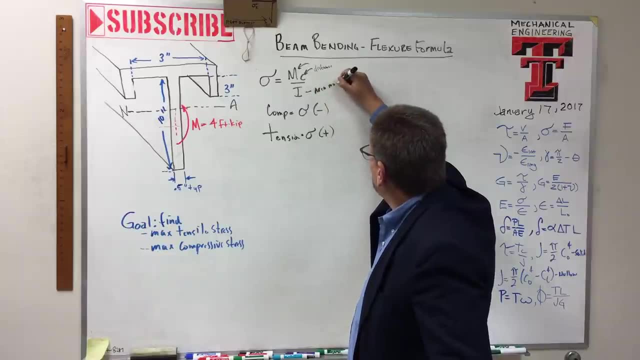 And then, of course, I. we learned I in statics, didn't we? I is the area moment of inertia, right, The MOI, okay, And what was the equation for that? Remember, we had to do the parallel axis theorem. The equation was I. 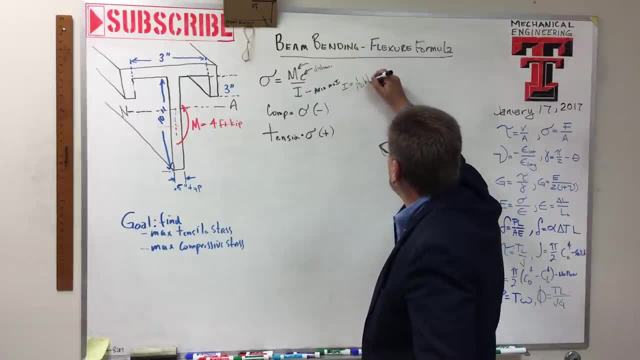 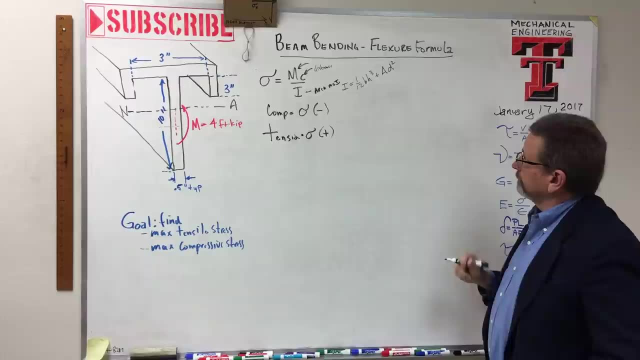 equals 1, 12 b h cubed plus a d square. excuse me, So that was the equation to find, I, for a rectangular shape. We're going to have to do it again. We're going to have to do it again, We're. 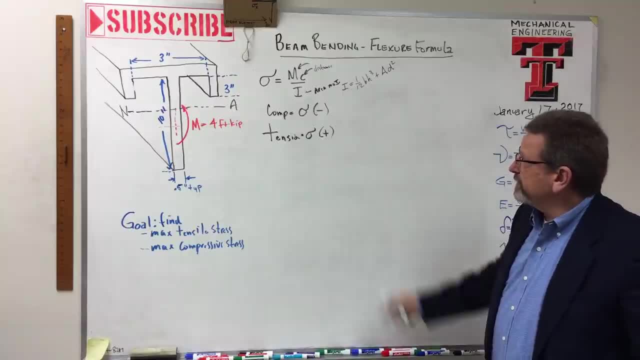 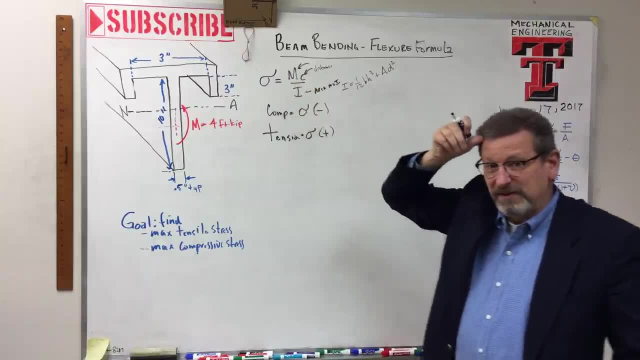 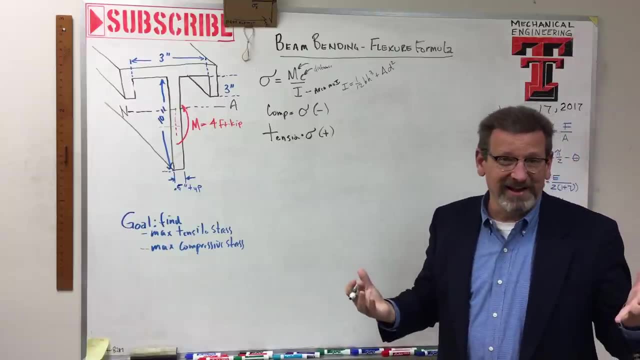 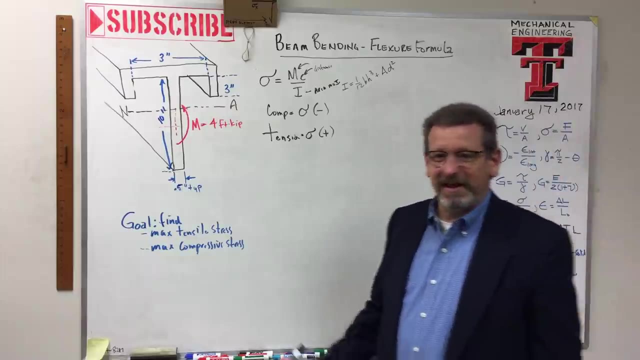 up. This is given. That's kind of given, except we don't have it here. So you know that neutral axis. where does it occur? It also occurs at what we call the centroidal axis. So step one for this problem: We've got to find the centroid of this, don't we y'all? So we're going back to statics. 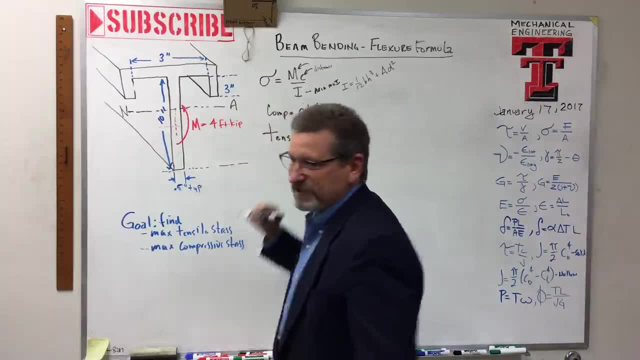 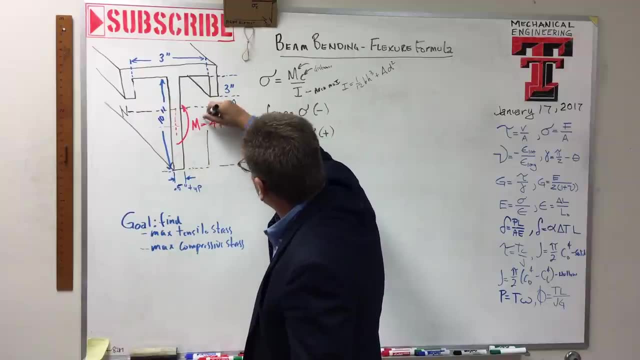 here and always start from the bottom of the part. I think that's easy. So if you just use the bottom of the part as a datum and find the centroid of the part, you're going to find the centroid of the part. So how far is it from the bottom of the part up to there? right, And that looks like it's in the 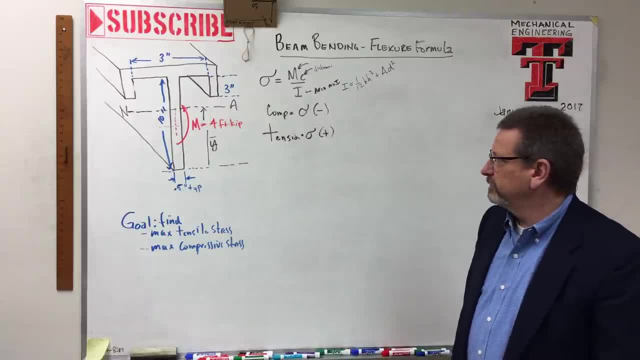 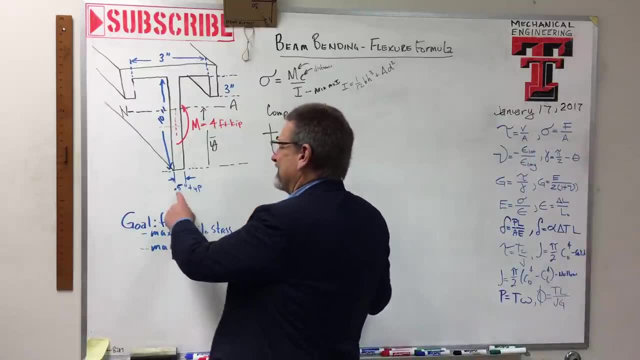 y direction. So we need to find y bar for this part. okay, How do we do that? We're going back to statics. Here we go. We're talking about a t cross section. This thing says it's 0.5 inches. 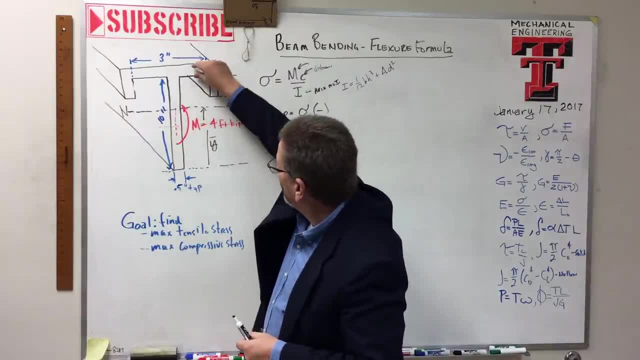 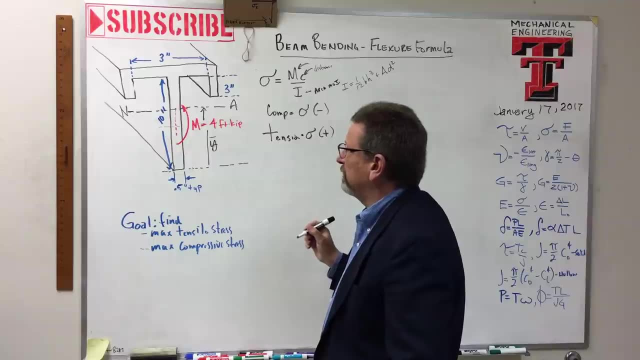 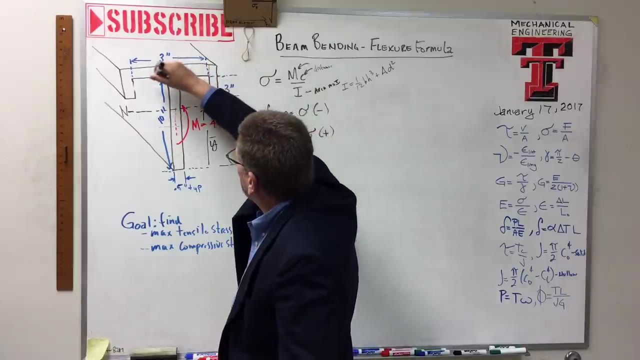 typical. What does typical mean? That means it's 0.5 there, 0.5 there, 0.5 there. The whole thickness is 0.5 everywhere. So what do you say? we divide this into- oh, I don't know. four shapes. right, Let's divide it here and divide it there. 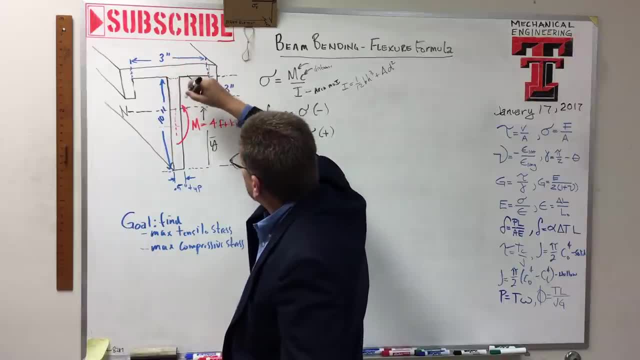 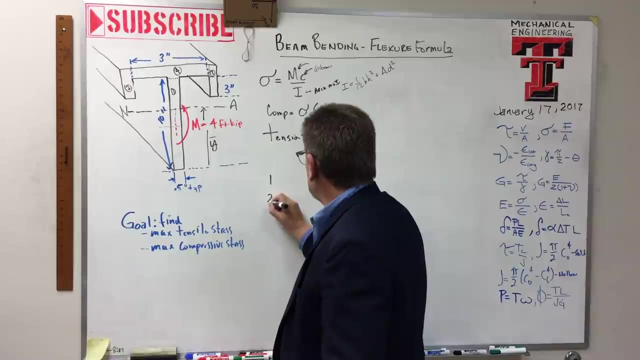 and we'll divide it across there, okay. So we'll call u shape 1,, shape 2,, shape 3, and shape 4, okay, So, if you remember from centroids, we're going to use our little table method. and here's the table method: Shape 1,, 2,, 3,, 4, right? 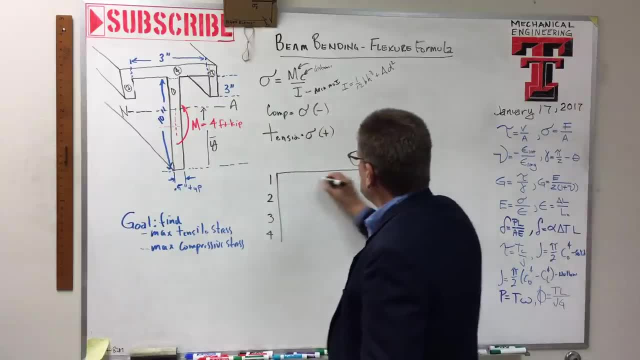 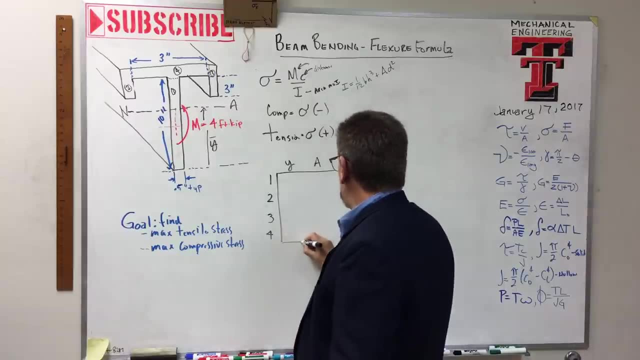 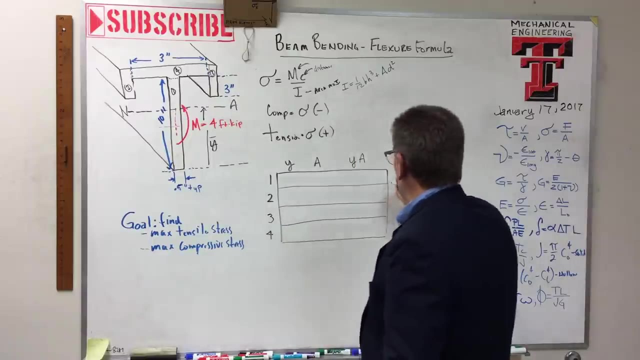 And then, on the top up here, what do I have? I have y, a and ya. okay, So all we have to do is fill in this little table here and we'll be good to go. okay, Because what is the equation? 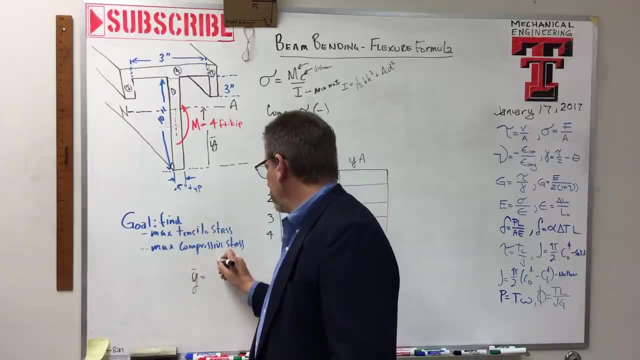 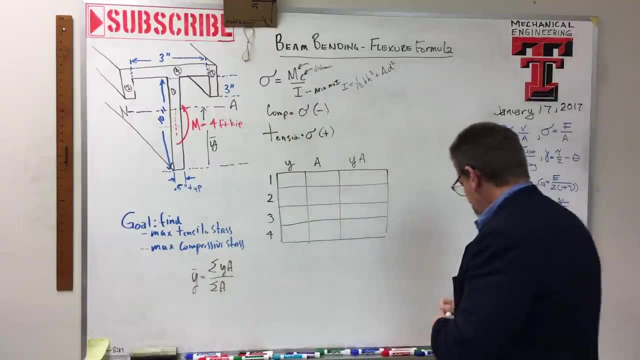 for y bar. y bar is equal to the sum of the ya's divided by the sum of the a's. Now y bar is бы, or y bar is equal to the sum of the y's and the areas right. Okay, 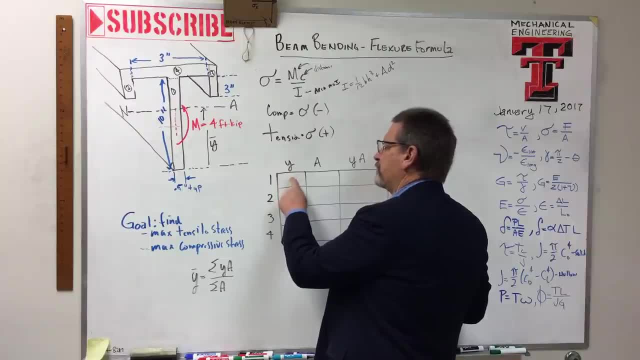 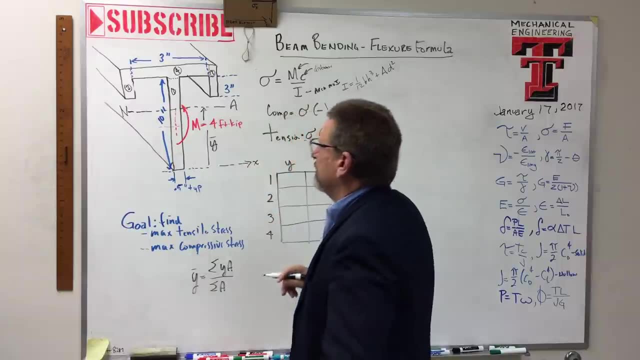 let me get this other black pen. it's working better. Here we go, So let's see if we can fill this in. Where is y bar for shape number 1,? okay, Now let's just call this 0 down. 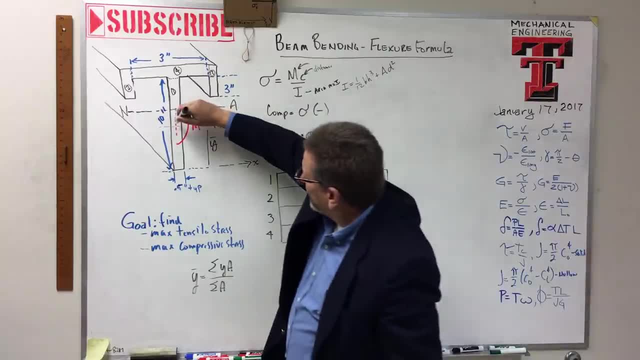 here. Let's just think of this as our x axis, okay, So this p shape number 1 is 10 inches tall, whereas y bar is right in the middle of that. so y bar is at 5 inches and the area of that is a 10 inch wide by 10 inches long, and that's zero. So they're both equal. Okay, So this y bar is at 10 inches tall and y bar is at 5 inches and the area of that is a 10 inches wide by 10 inches long, and that's 0.. 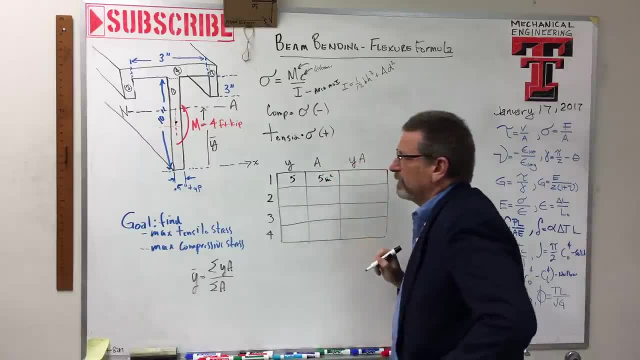 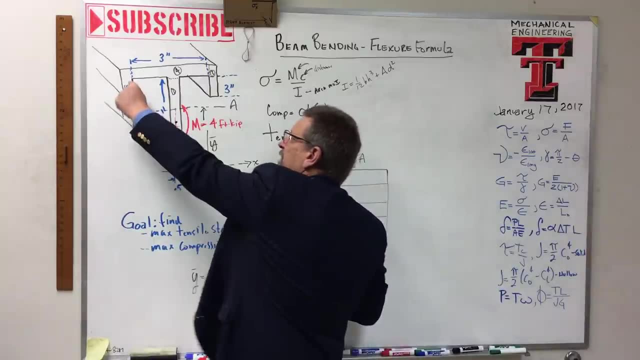 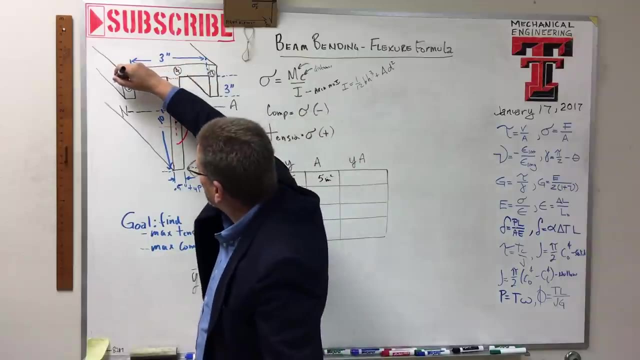 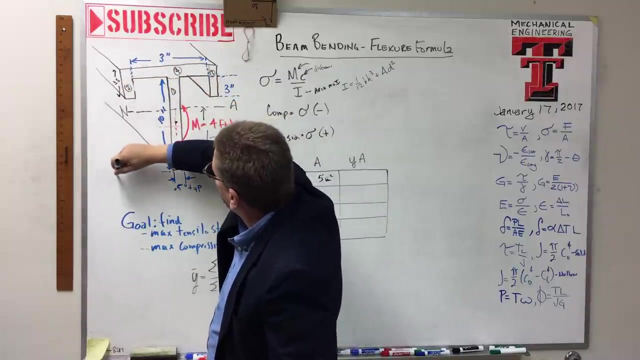 so that's five inches squared right, okay, and then shape number two. where's shape number two? he's way over there. where is y bar? well, this is three. so the whole thing is three and a half, isn't it? this is 3.5, okay, and how far is it from the bottom to the top of the part? 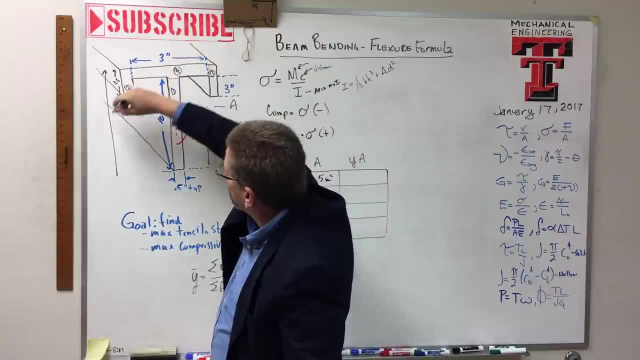 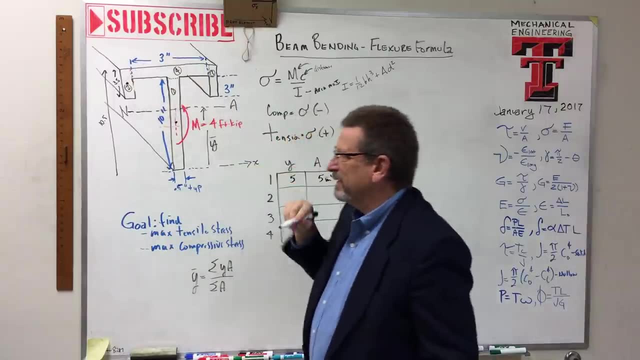 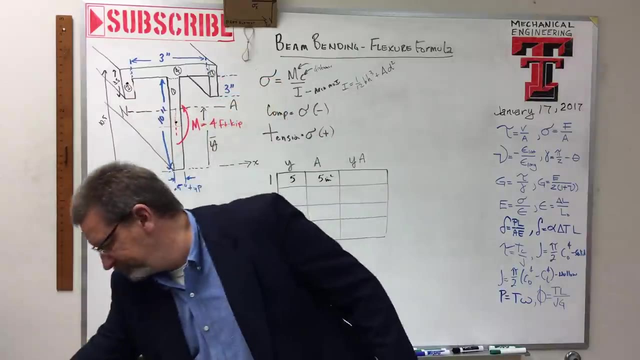 well, that's 10 plus a half, so that's 10.5, right? so where is y bar for this guy right here? well, you got to go 10.5 and then come back half of 3.5, right? so here we go. i'm using my. 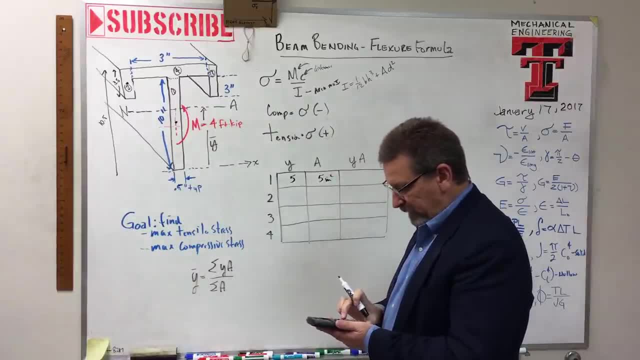 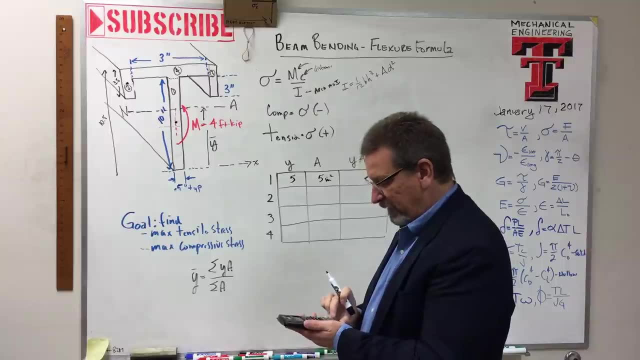 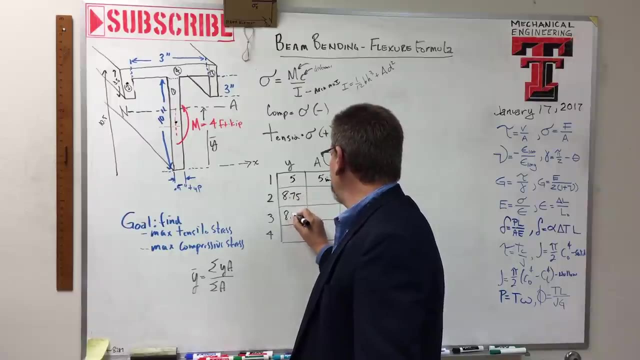 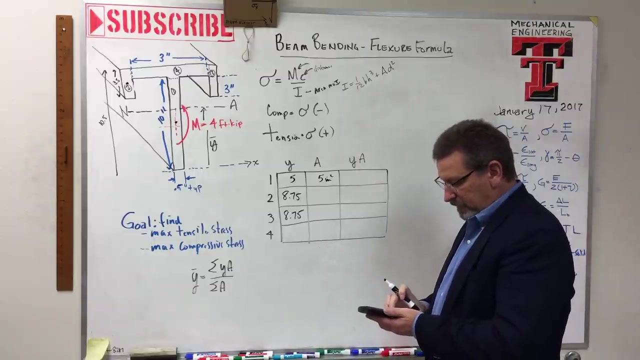 don't make a mistake on: 3.5 divided by 2 equals 1.75. so 10.5 minus 1.75 is 8.75. is that what y'all got? and this one's also 8.75. now the area for those is 3.5 divided by 2. 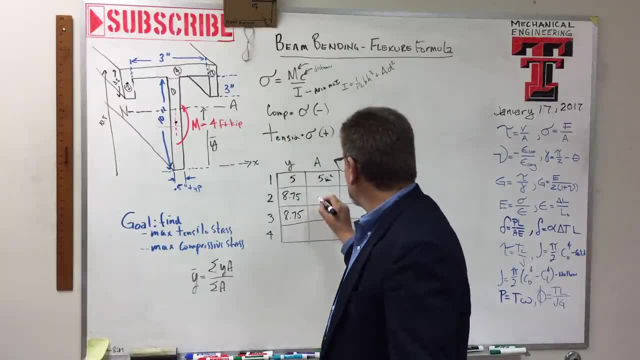 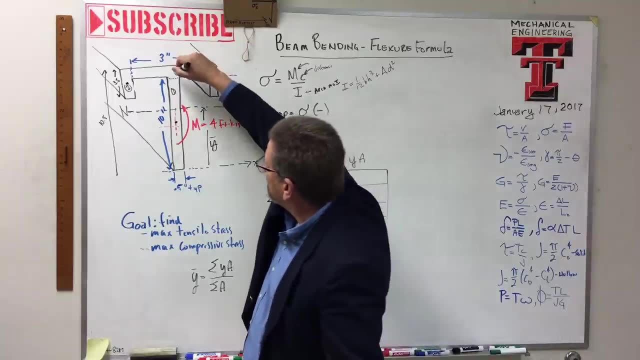 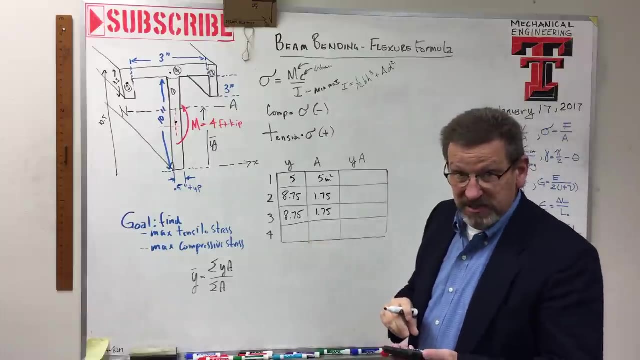 right, or 3.5 times a half wide, so that's 1.75. and finally, shape number four: where's the centroid of this guy? from the bottom it's 10 plus a half of a half right, so 10 plus 0.25, which is 10.25. 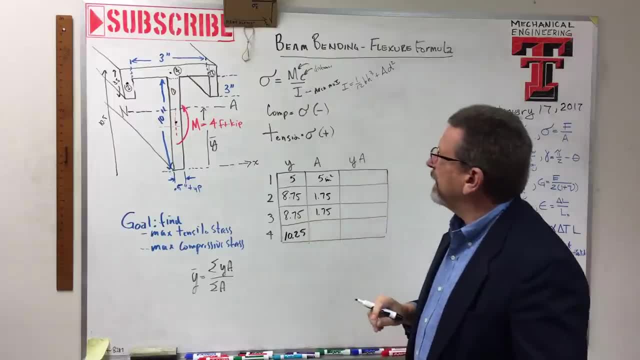 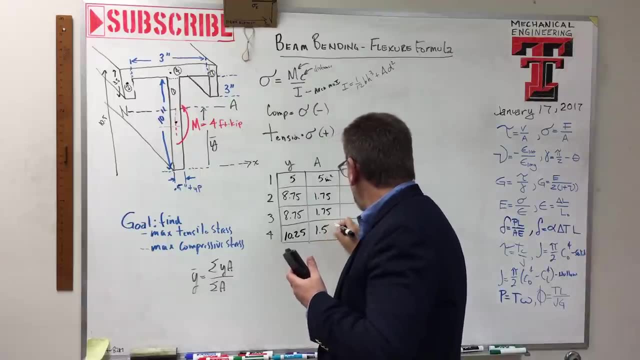 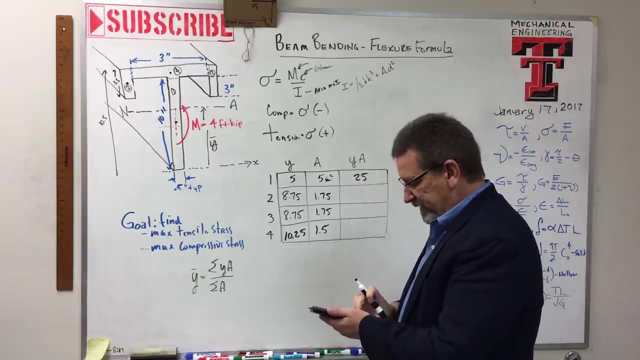 and the area of that guy is three times 0.5. i'll do that one, one and a half, okay. so we need to fill in y times a, so that's 25. what's this one? 8.75 times 1.75 equals 15.31. 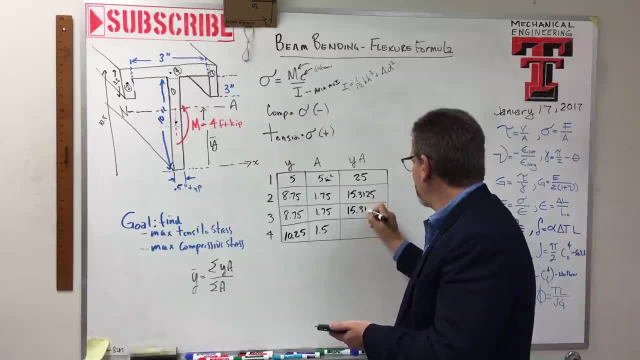 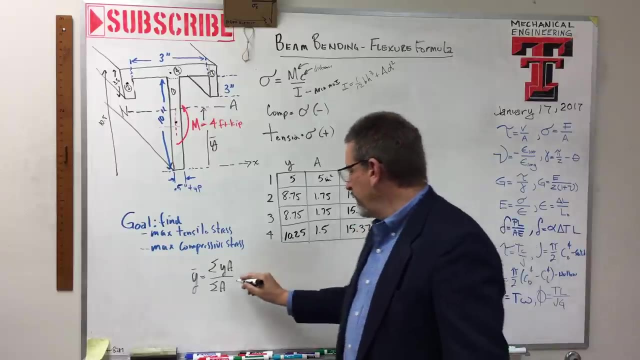 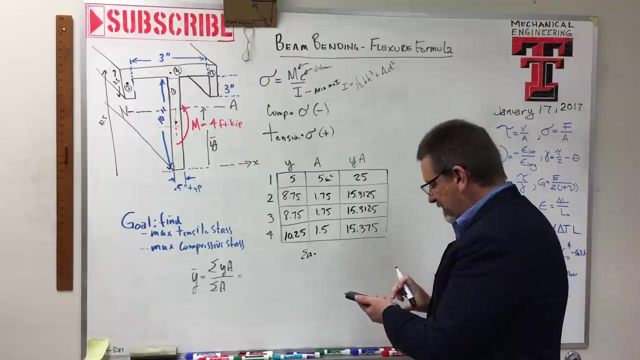 and this one is same and this one, 10.25 times 1.5, equals 15.375. okay, i think we're almost there, so we need the sum of the a's. well, that's going to be right there, isn't it? the sum of the a's is 5 plus 1.75 plus 1.75. 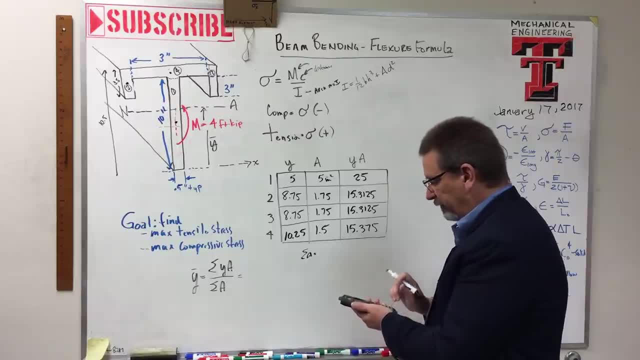 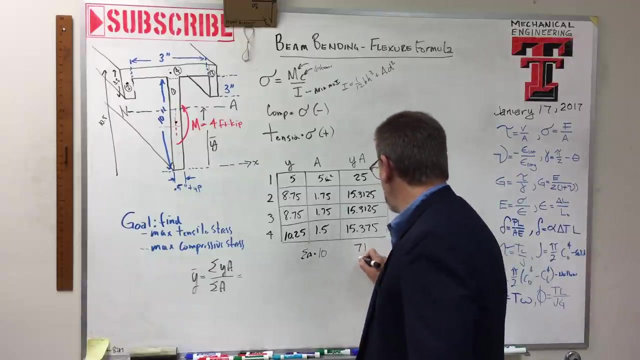 plus 1.5 equals 10, and then we need the sum of the y a's, that's 25 plus 15.3125 times 2 plus 15.375 is 71. okay, so what is y bar? it's 71 divided by 10, which is: 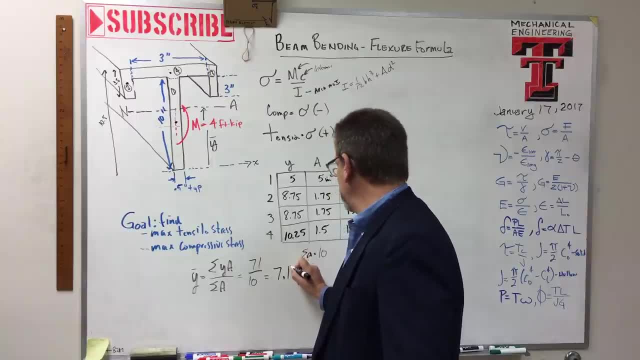 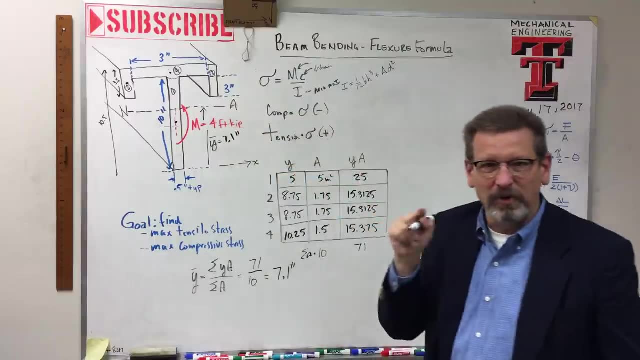 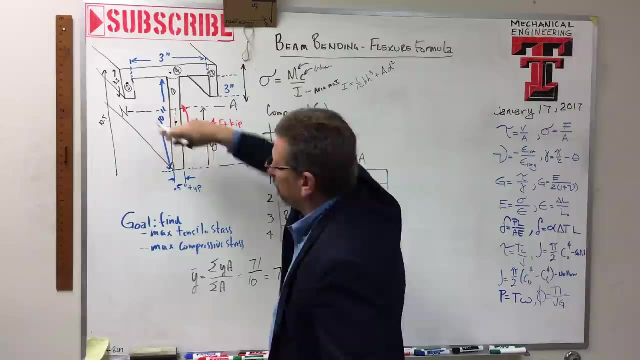 7.1, and these are in inches, aren't they? so y bar is 7.1 inches. that neutral axis is 7.1 inches from the bottom of the part, which means that from the top of the part right, the whole thing was 10.5. 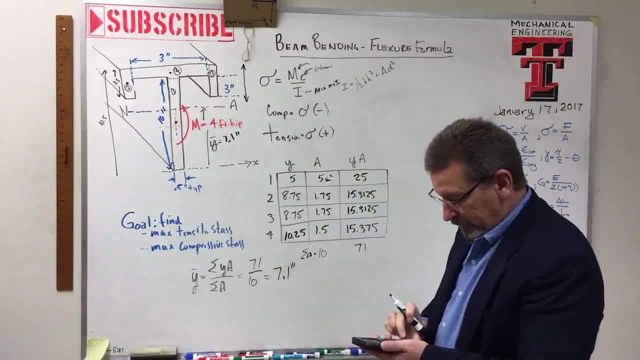 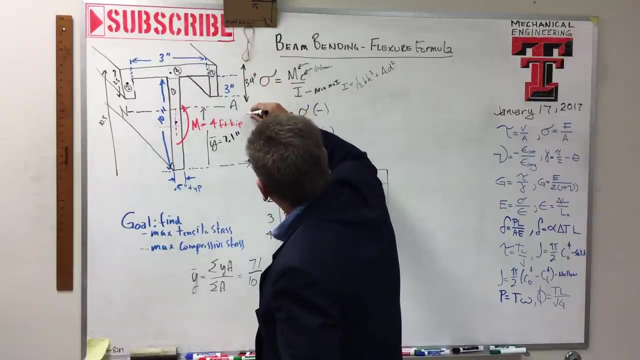 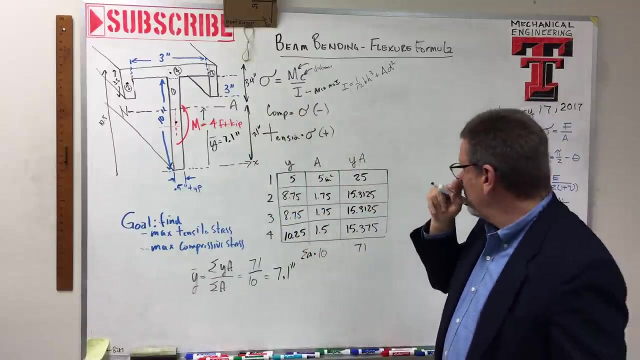 so 10.5 minus, oh no, clear. 10.5 minus 7.1 is 3.4. so this right here is 3.4, okay, and then over here, 7.1. that's step one, right? we don't even know anything about that. we know where the neutral axis is. 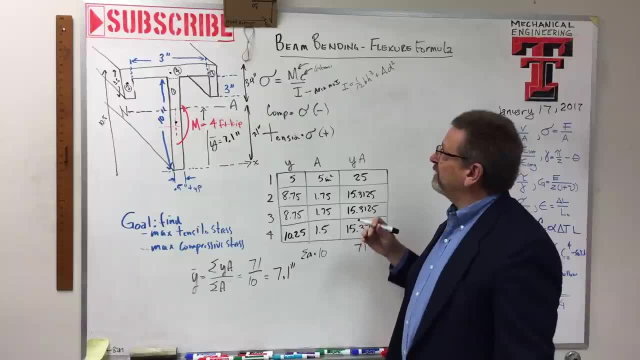 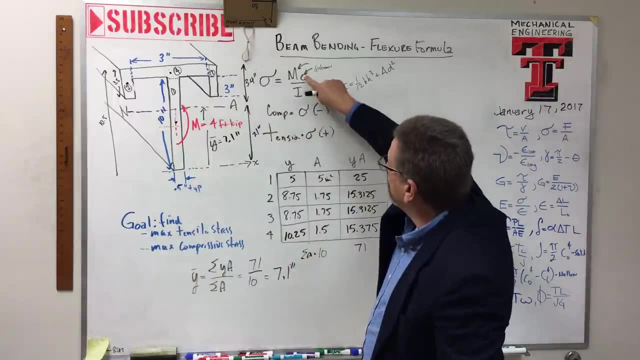 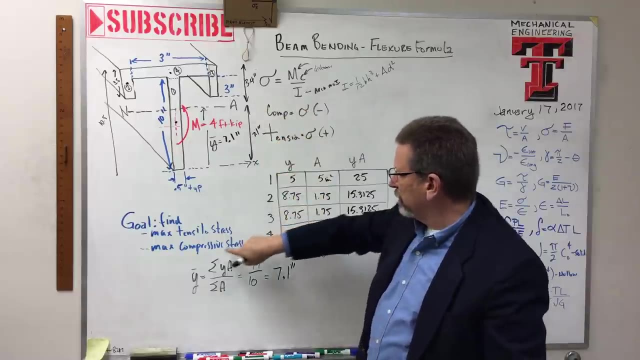 we had to find the neutral axis, matter of fact, for tensile stress right, the part that's in tension, which is the bottom. what is c going to be? what is the distance? 7.1 from the neutral axis to the bottom? is 7.1 for compressive stress, which is the top? what's c going? 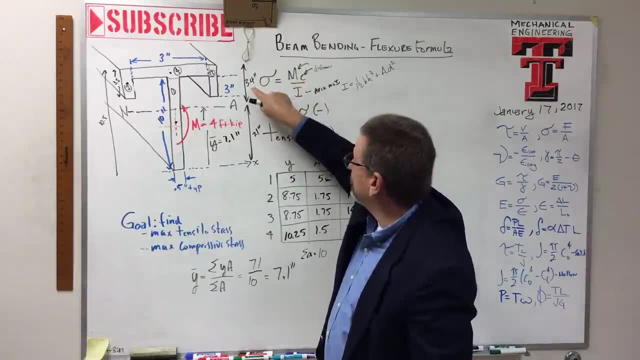 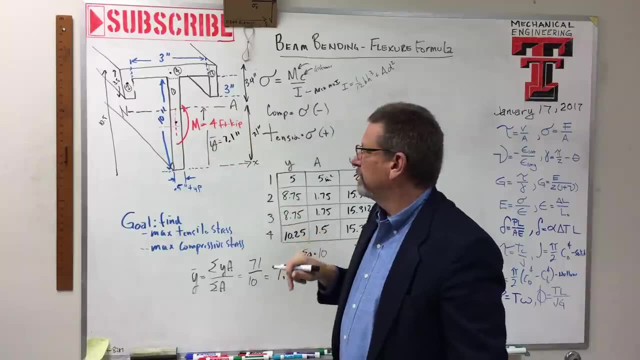 to be from the neutral axis to the top. that c is going to be 3.4. so we did kind of find something for our equation there. now the moment is already given and we're going to have to be careful because that's in foot kips and all our stuff is in inches. so that's another trick there. 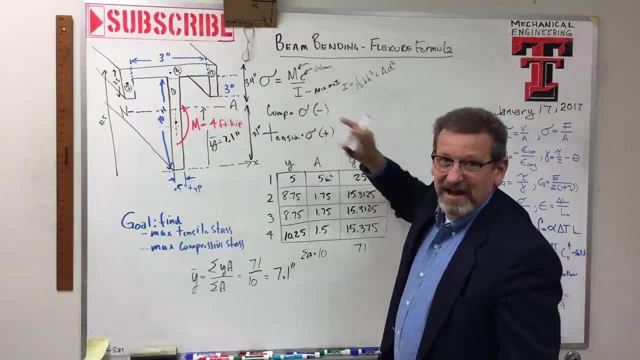 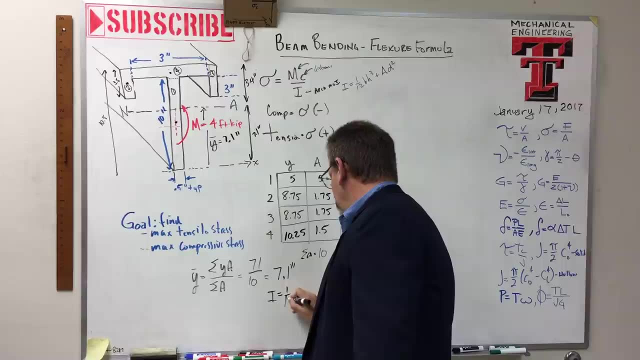 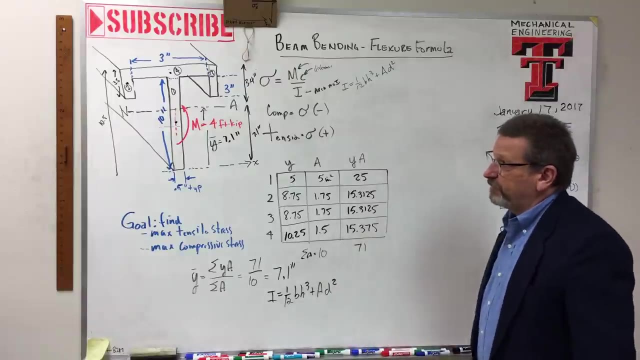 um, i think the last thing we need to do, let's calculate i. if we calculate i, i think we're going to be there, okay. so i say: i equal to 1. 12th馬 equals one twelfth bh cube plus ad squared. so since we have this in four parts, let's 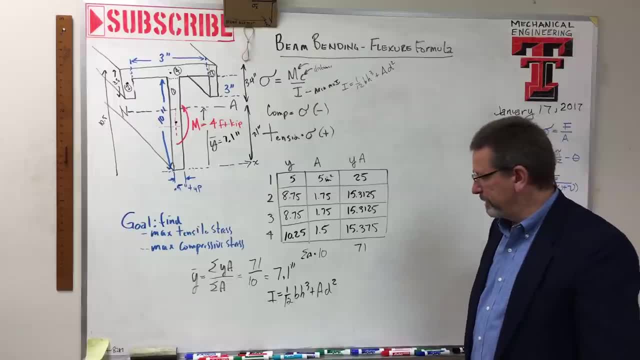 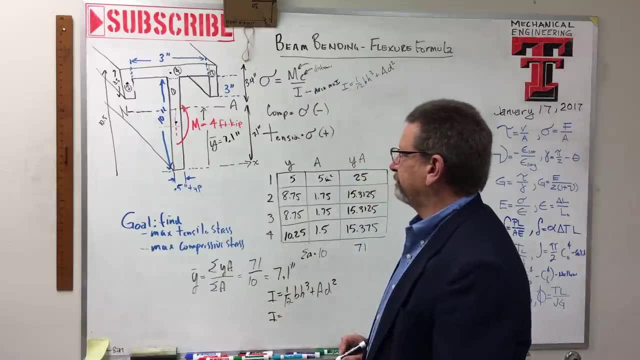 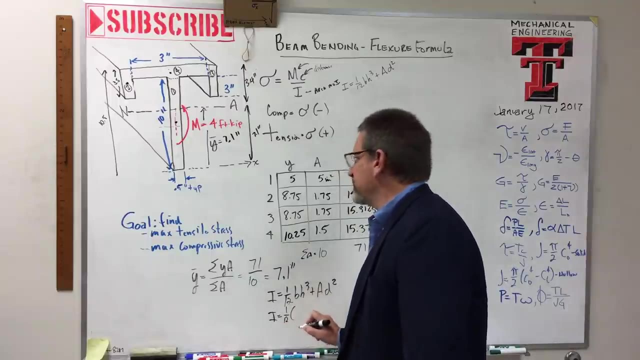 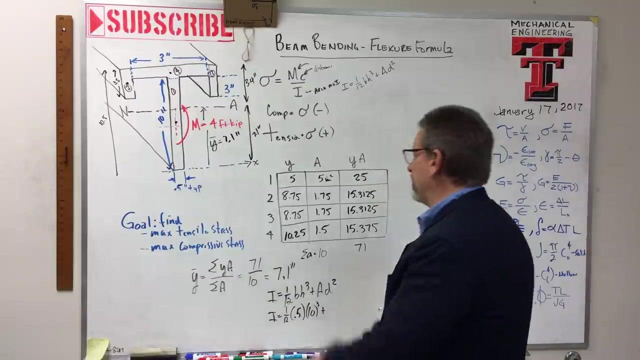 just do this in four parts. okay, we'll find i in four parts. okay, so let's do piece number one. okay, piece number one. oh, my is one. twelfth the base. what's the base? point five, what's the height? 10 plus the area of piece number one. this is nice. we already have that. 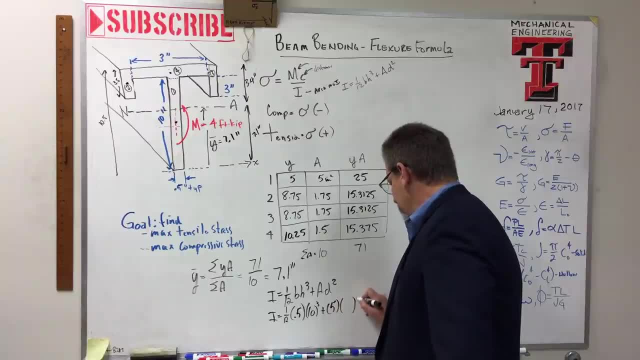 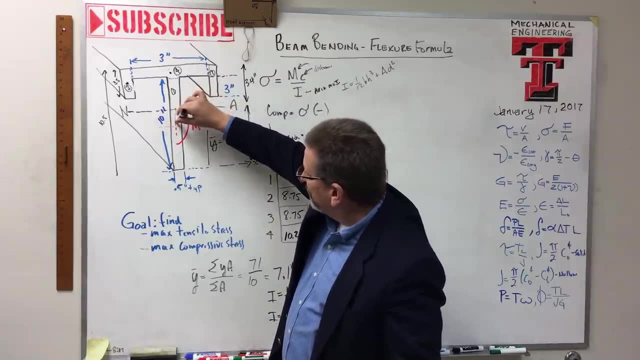 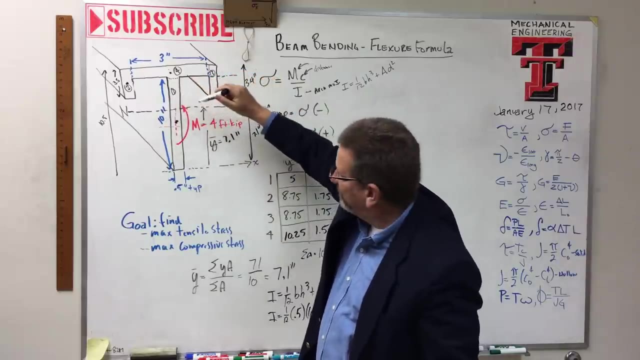 plus five times. here's where most people mess up is what is d? remember? the d is the distance from the neutral axis of the whole thing to the centroid of the part that i'm working with. so i'm working with this piece here, so this piece here is in the middle of this 10, right? so i go. 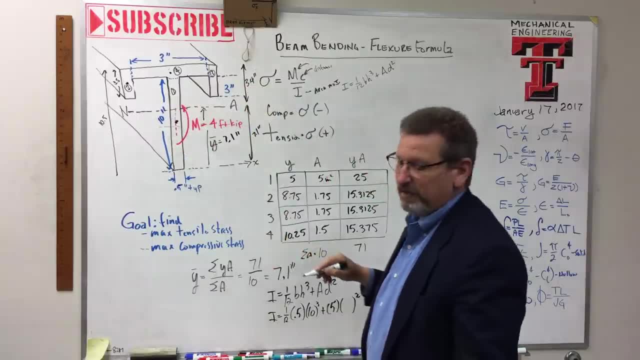 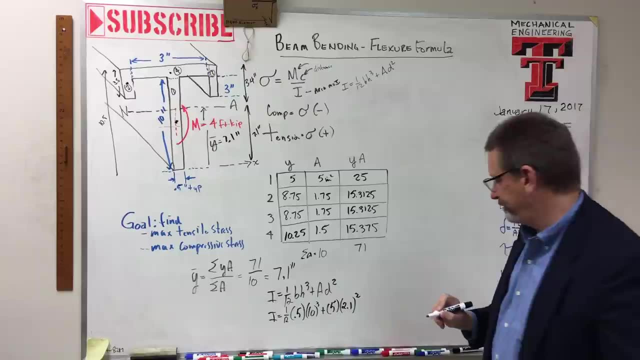 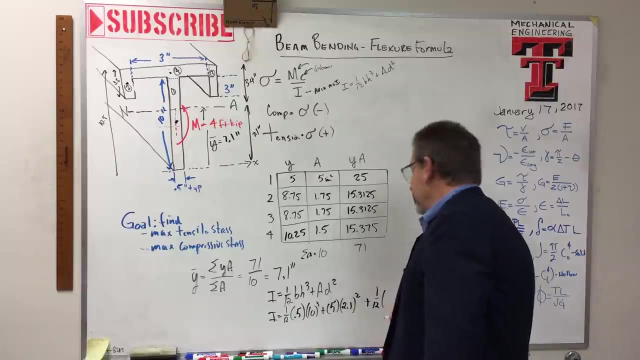 to the outside of the part 7.1 and i come back five. so that means that the d here is 2.1. okay, that's piece number one. okay, so let's do piece number two. so plus one. twelfth, what's the base on piece number two? this little guy? the base, half the height, 3.5 plus the area. 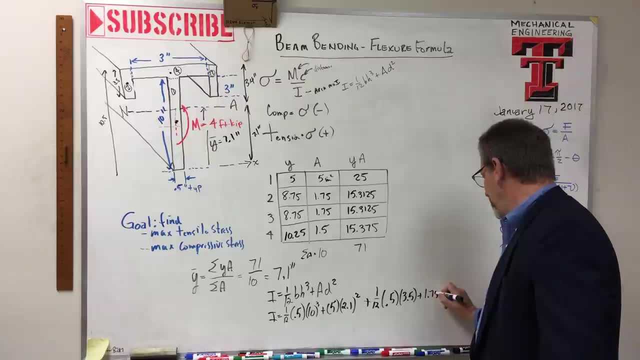 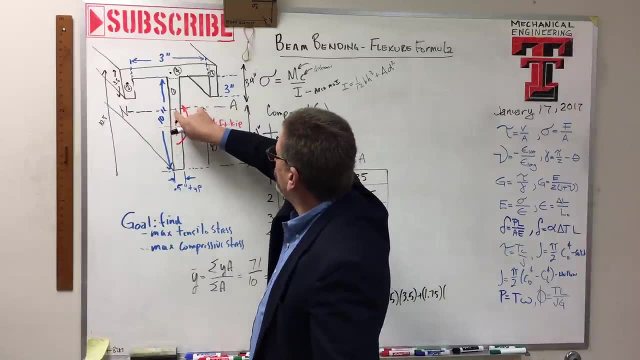 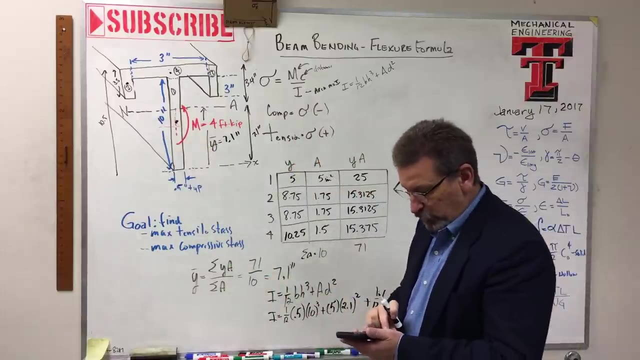 the area is 1.75. and then what is d remember? d is if i go from the neutral axis to the outside of the part, that's 3.4, and then i come back half of that 3.5. so 3.5 divided by 2 equals no 3.5 divided by 2. 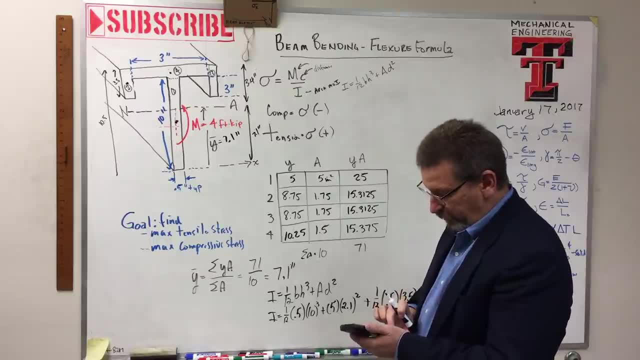 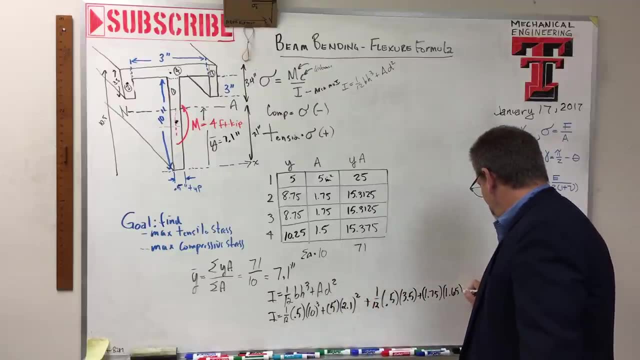 is 1.75, and so 3.4 minus 1.75 equals 3.5. divided by 2 is 1.75, and so 3.4 minus 1.75 equals 1.65. okay, now, that's piece number two. there's piece number one. there's piece number two. 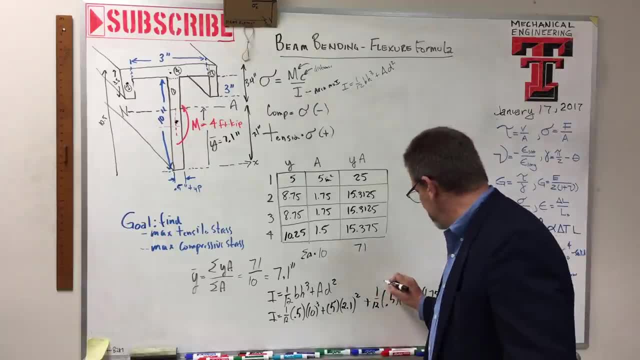 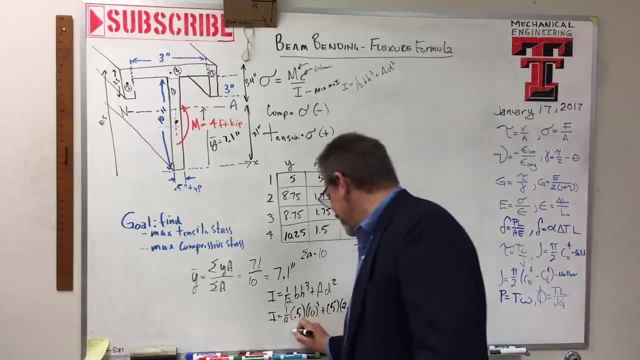 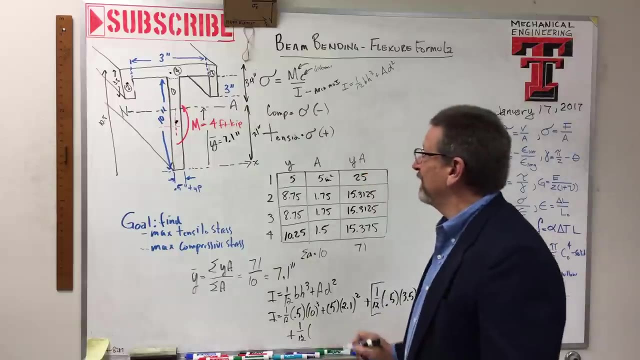 is piece number three the same as two, yep, so let's just do this, let's toot them's that, let's put a two on there times two, and then we have one more plus. last piece is piece number four, there at the top. so we got one twelfth. the base is what? three? 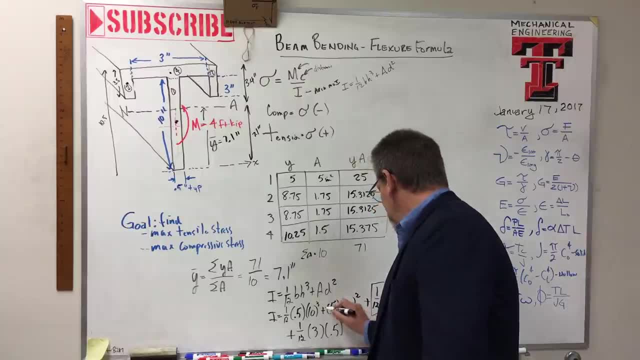 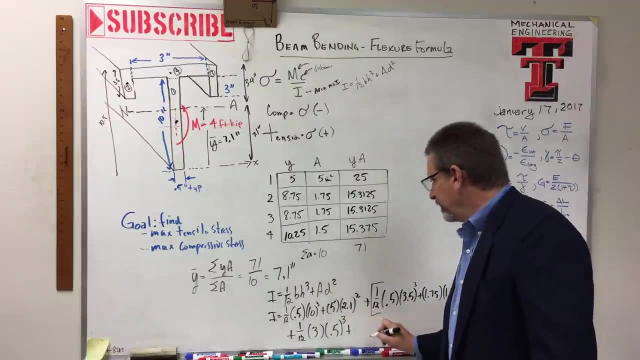 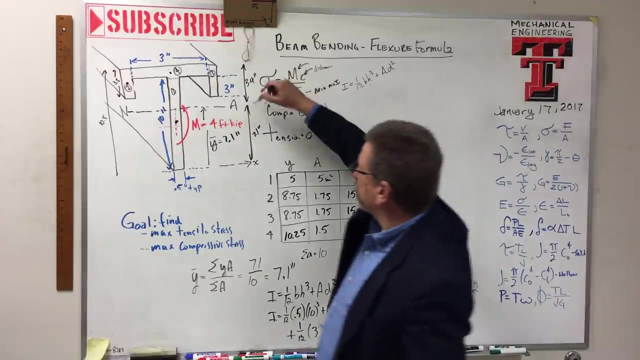 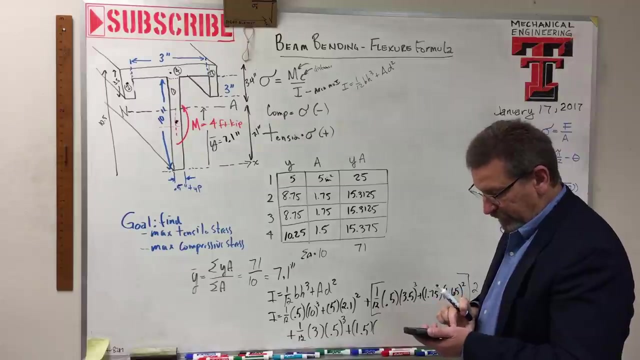 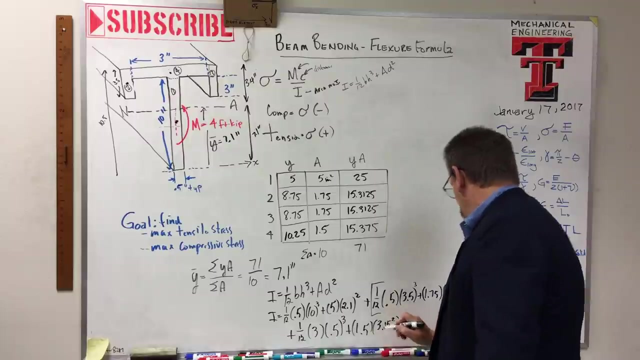 the height. this time is point three point five b blade, plus the area which is one point five times d. well, d is 3.4 minus point four minus .25, right? so three point four minus .25 equals. okay, that's one, three point five And that's squared. 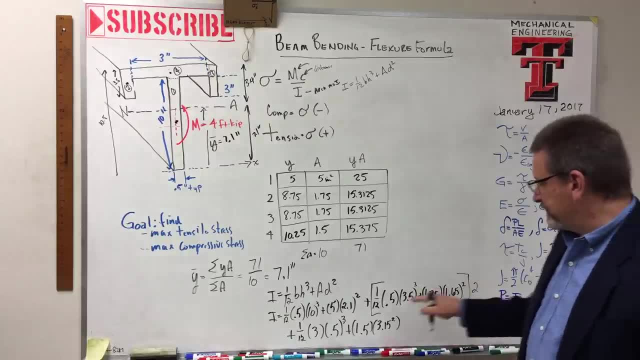 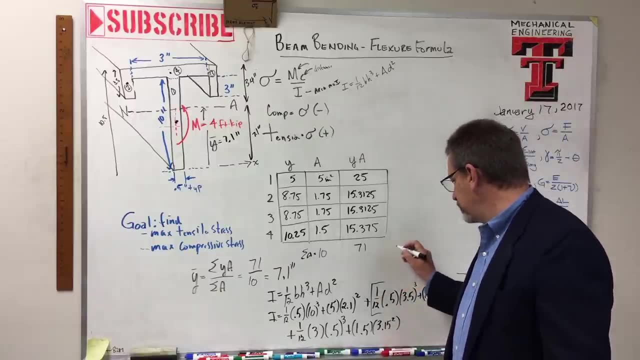 So now what we've got to do is put all this in our calculator, okay, And this is going to give us? what is this going to give us? This is going to give us inches to the fourth. okay, So I'm going to put these in my calculator: piece 1,, 2,, 3, right. 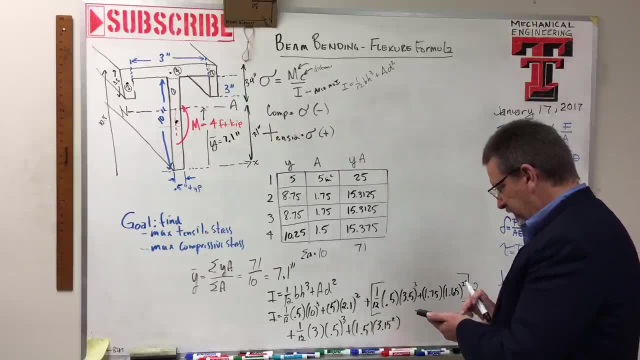 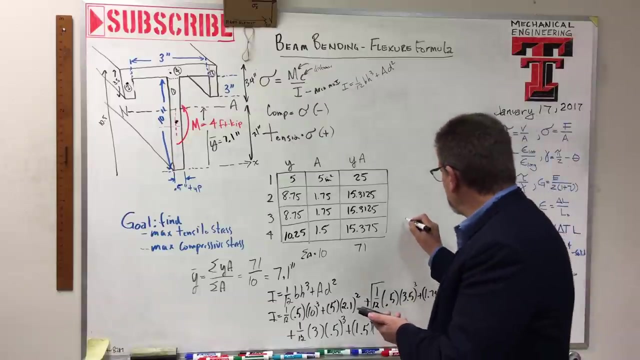 So here we go. Let's see if I can do this. 0.5 times 10 cubed equals. divided by 12, equals 41.67. plus 5 times 2.1 squared equals okay. So the first part is 63.72.. 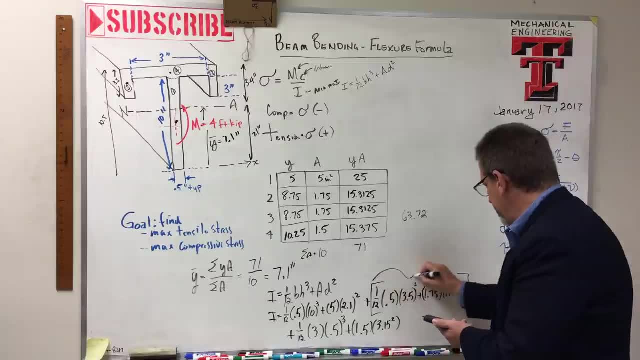 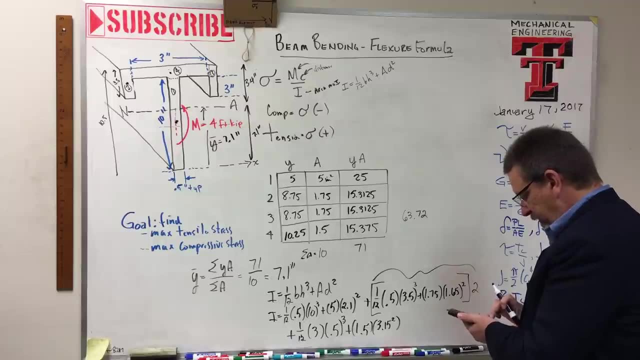 That's what that is. Now I'm going to do this piece here, this chunk here. Okay, And that's 0.5 times 3.5 cubed, equals divided by 12, equals plus 1.75 times 1.65 squared equals 6.55.. 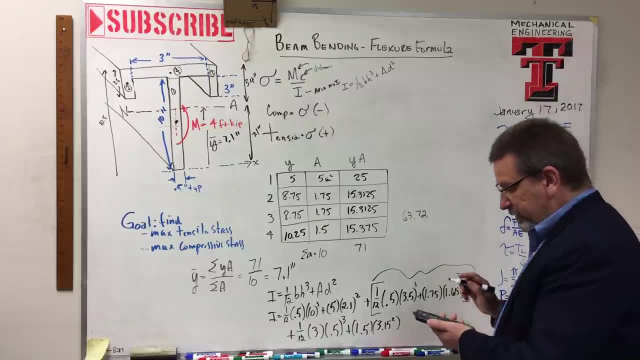 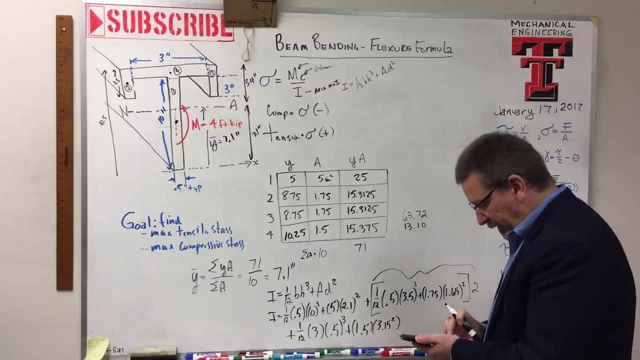 And then I'm going to multiply all that times 2.. So that's 13.10.. Now I'm going to do this last piece down here: 3 times 0.5 cubed equals, divided by 12, equals plus 1.5 times 3.15, squared, equals 14.92. 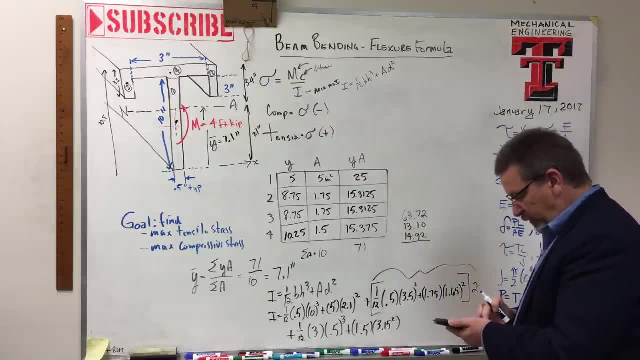 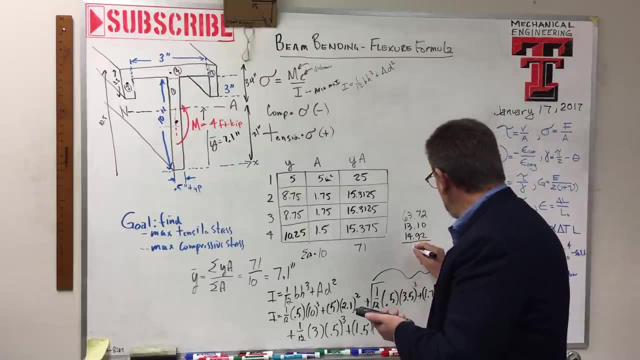 So I'm going to add all those together. So plus 13.1 plus 63.72 equals 91.74 inches to the 4th, And that is what I about bending around the x-axis is equal to okay. 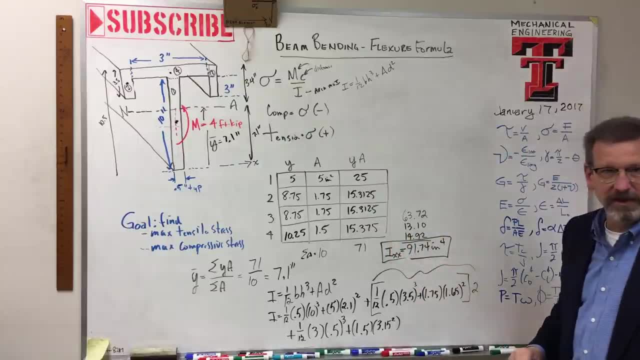 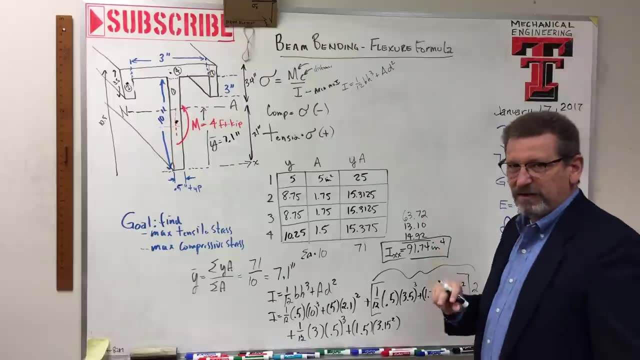 So that is a lot of work for the moment of inertia. okay, This should be a statics review. If you don't understand how to do this, go back to statics- the very last 3 or 4 videos in my statics series and review that stuff, okay. 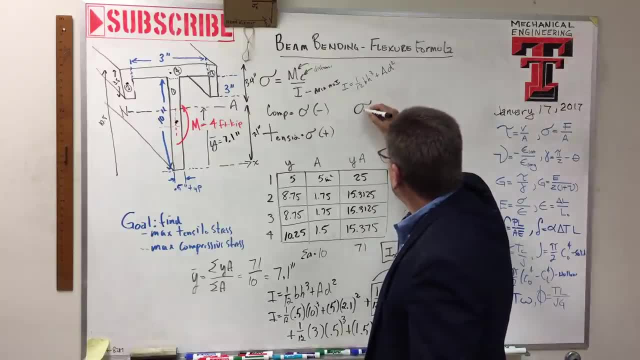 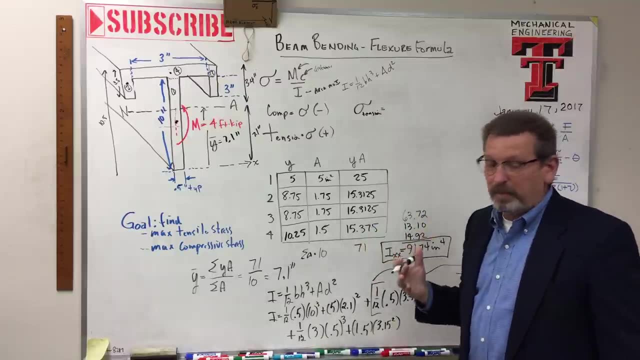 So here we go, Sigma. Sigma And for tension is equal to for tension tension's, where The top or the bottom, The bottom right, It equals 4.. I'm going to do this equation here, MC over I. 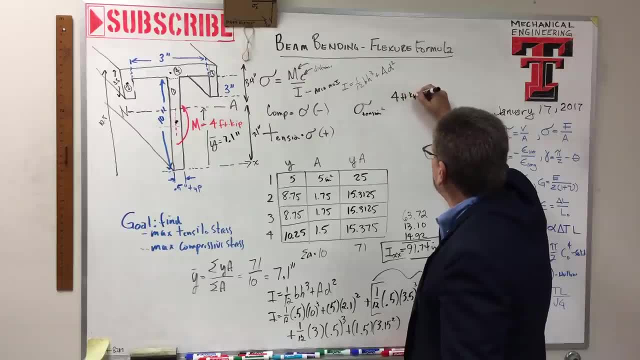 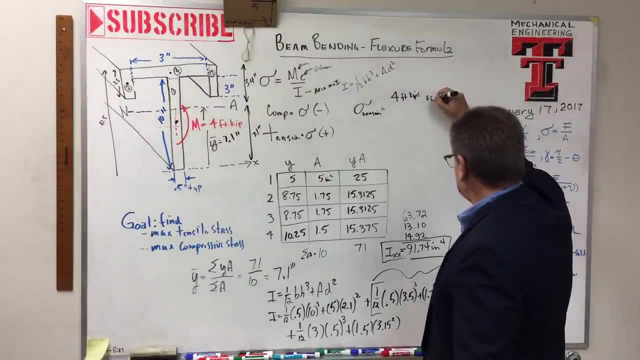 So 4, and that's foot kips. Remember, a kip is 1,000 pounds, But we don't want that in feet, do we? So 1 foot is 12 inches, right? That way our feet will get canceled out. 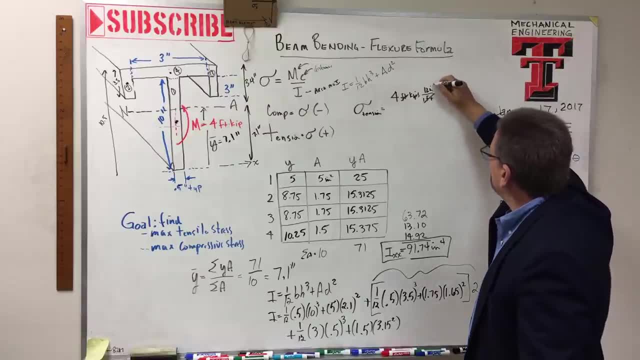 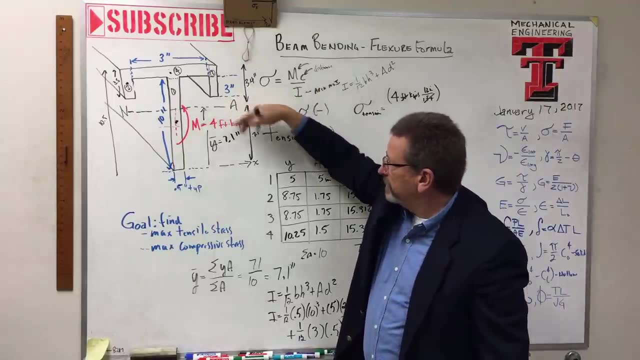 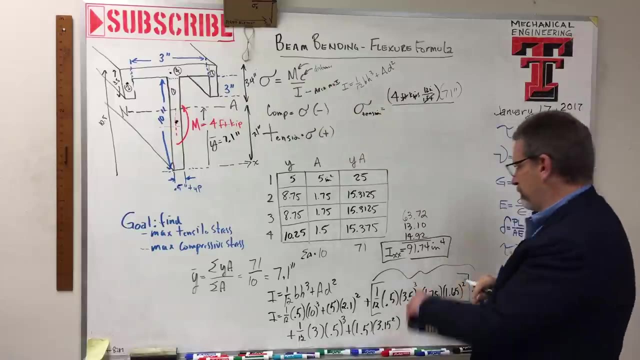 And what is that going to give us Times? what M times C? And what's the distance? C is for the bottom of the part, for tension, So C is going to be 7.1 inches divided by the moment of inertia, which is 91.74..